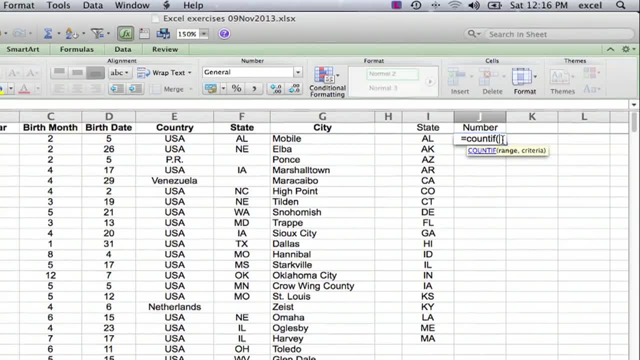 So we have COUNTIF and the first thing, the first argument, in other words, the first entry in the function is the range, which is the range that we want to count. So I'm going to go over here and I'm going to select all of the entries in column F. 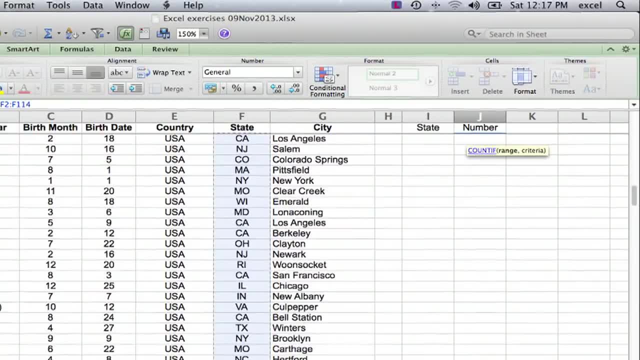 So I just start at the top and drag down until I get to the bottom. Just bear with me. we're almost there and now we're done. Whoops, we went a little too far. There we go all the way to the end. 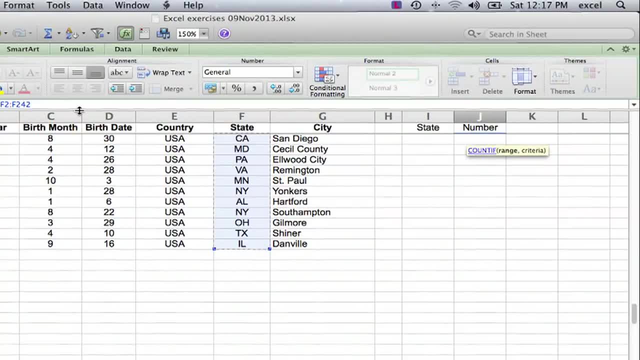 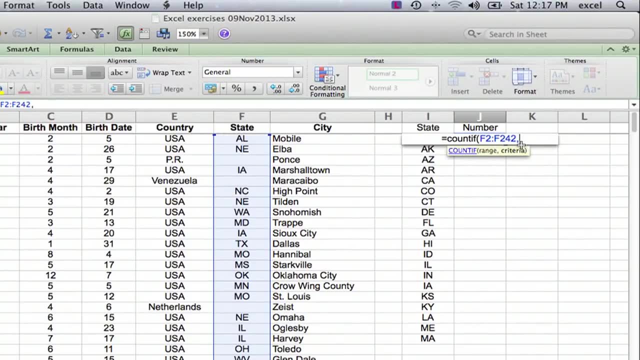 Now I'm still in edit mode in my formula, if you look up here, And we go all the way to the top and now we type a comma and the next entry is criteria. Criteria is going to be the state, which is the entry in column I. 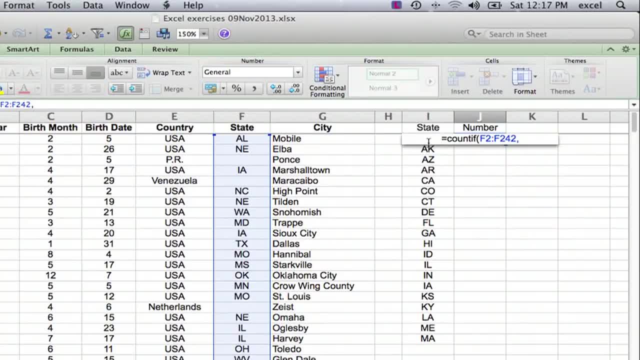 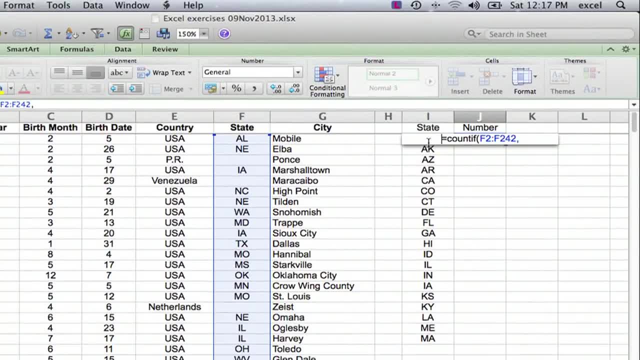 It's got my formula bar over the place where I want it to be, So I actually have to manually enter in cell I2.. So I'm just going to type in I2, and then I'm going to type a close parenthesis. Whoops, I got the entry in the wrong place. 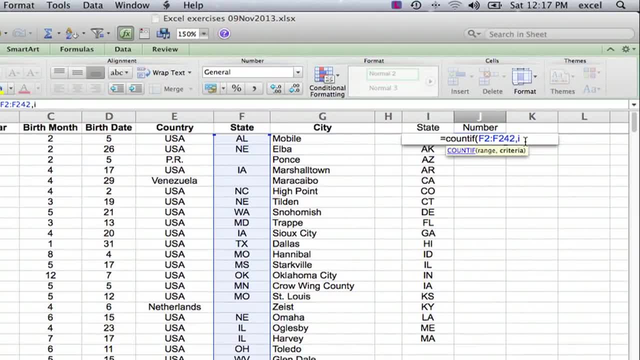 I have to put my cursor over here and I'm going to type in I2, close parenthesis and hit a return, and there we go. So Alabama, AL. there are 12 entries from Alabama. Now what we want to do, of course, is copy that formula down to all the others. 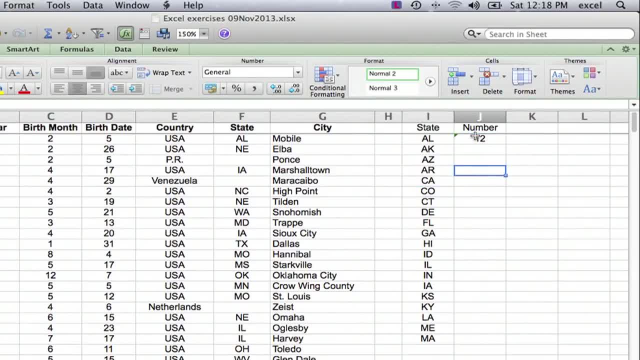 Now, what we want to do, of course, is copy that formula down to all the others. Now, what we want to do, of course, is copy that formula down to all the others. But before we do that, we have to make sure that when we copy the formula- as you may know, Excel, when you copy a formula changes all of the relative references of the cells, So we want to prevent it from doing that. We want the range here up in my formula bar. we want the dollar signs before all of the row numbers in, just the range here. 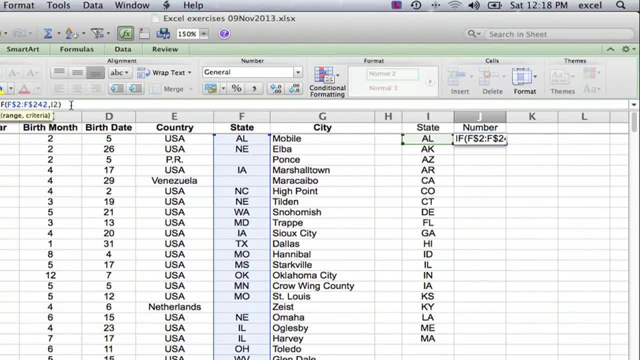 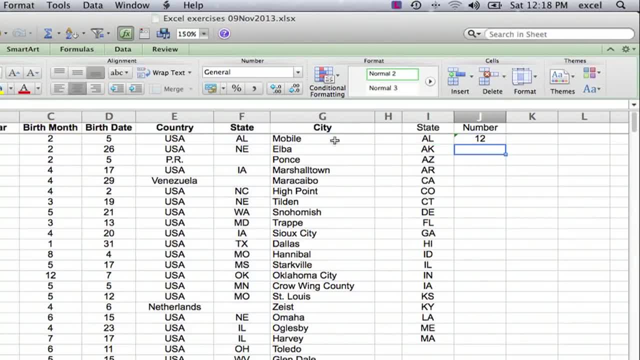 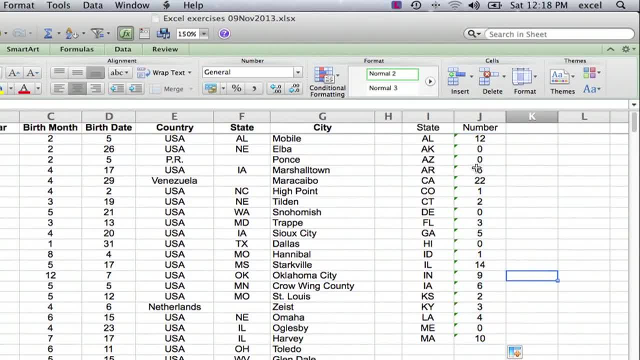 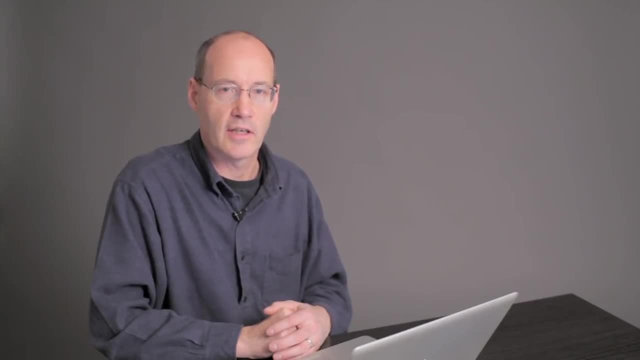 it's going to copy that formula to all the other states and, sure enough, this is the number of entries in column A for each of the different states. So I hope this has been helpful. I'm Ted count the number of occurrences of an entry in a range in Excel. Thank you for watching.